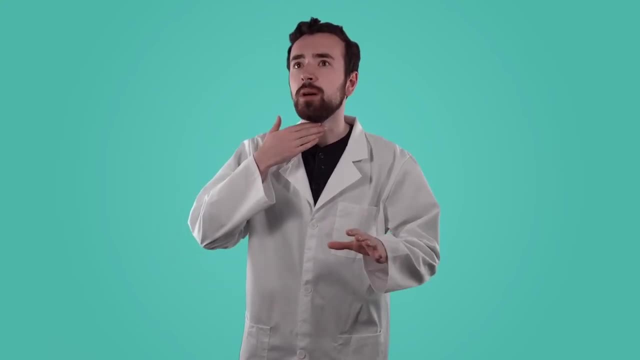 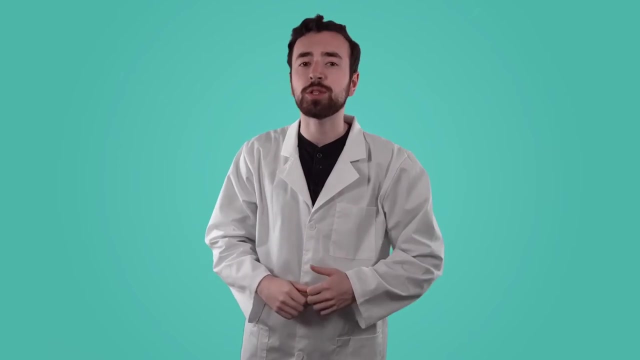 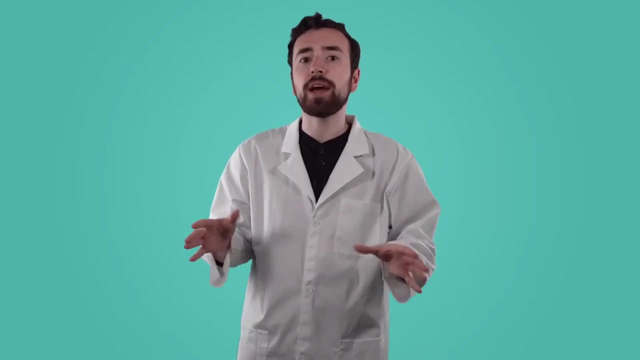 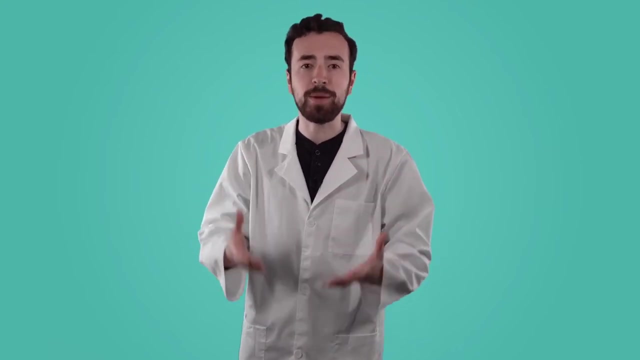 put your hand against your throat and hum. What do you feel? Pause the video here and describe your observations in your guided notes. No matter your level of musical talent, you should have felt a kind of buzzing feeling in your throat. That's vibration. Ears sense sound energy by being very sensitive to vibrations. When a 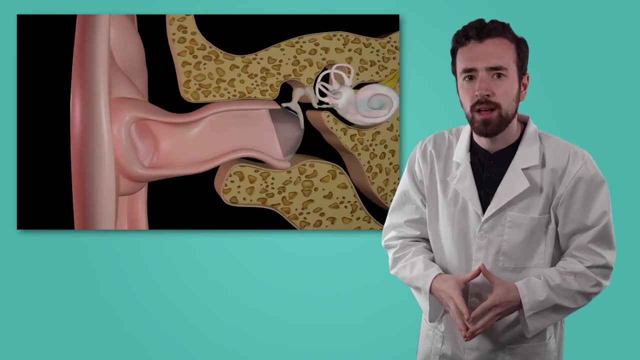 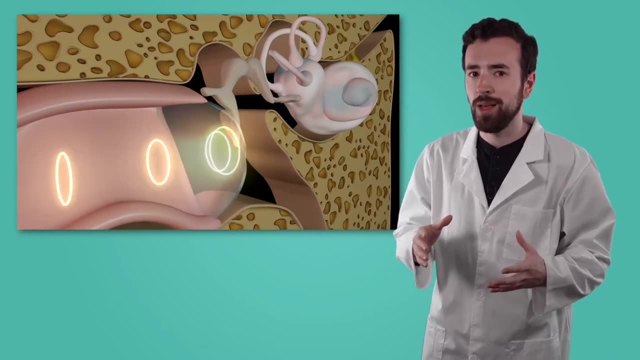 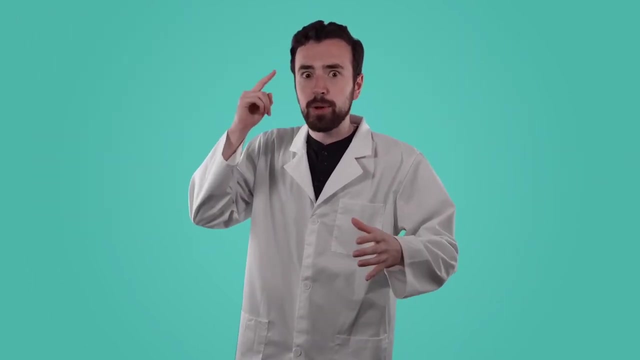 sound reaches your ears, like the sound of my lovely voice. the vibration causes a special part of the ear called the eardrum to vibrate as well. The vibrations in the eardrums are the signals that send signals to the ear to make a sound. We can make sound sounds through 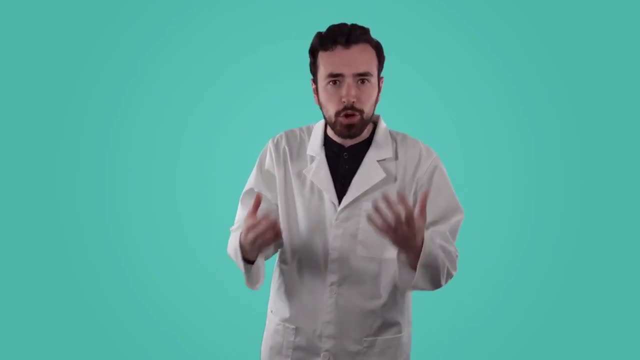 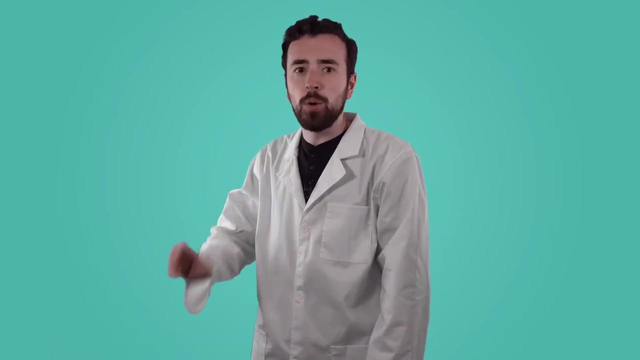 our heads, From the mouth, from the ears or the ears to the ear drum. it's a reaction that sends signals to your brain saying: hey, brain, listen up, there's a sound here. Your brain then interprets the sound, deciding if it was a barking dog, a car alarm or the ice cream truck driving off before I had a chance to get my money. Hey, wait. Sound energy is vibration and our ears allow us to sense the vibration and vibration That's vibration. We're talking about the sounds of our ears and the sounds of our ears. If you feel that you're. 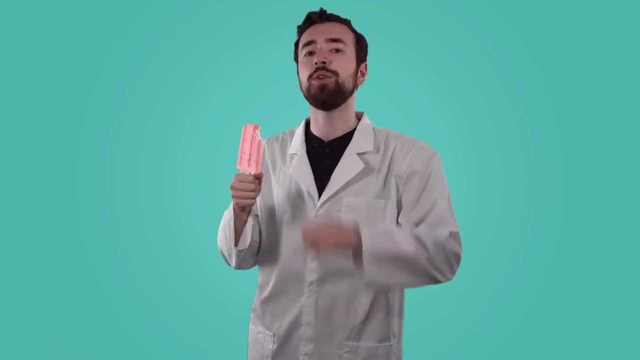 hearing something. or you're able to hear something, or you feel like you can catch it. that means you know the sound, But then you can't hear that word. That's vibration. It's vibration. That's vibration. sense those vibrations providing us with an important way to interact with our world. 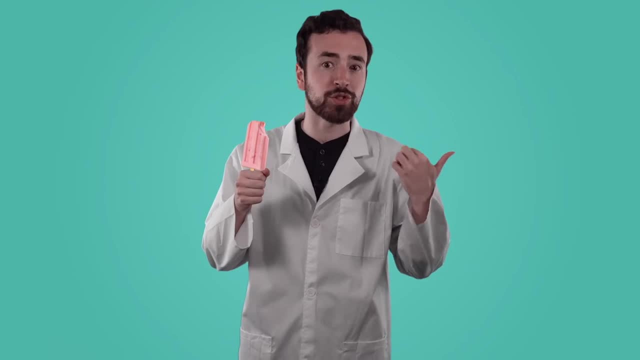 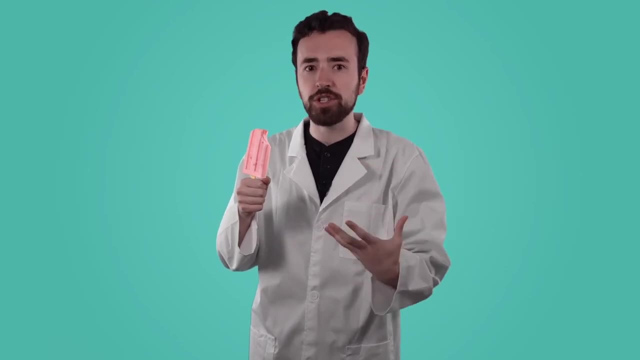 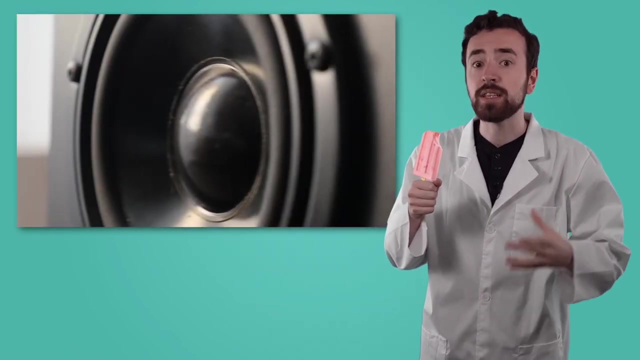 But how did the vibrations coming from the truck down the street get all the way to my ears? Well, sound energy travels as vibrations moving through matter. Let's take a look at what that means. To create a sound, the speakers on the ice cream truck vibrate. That movement causes the 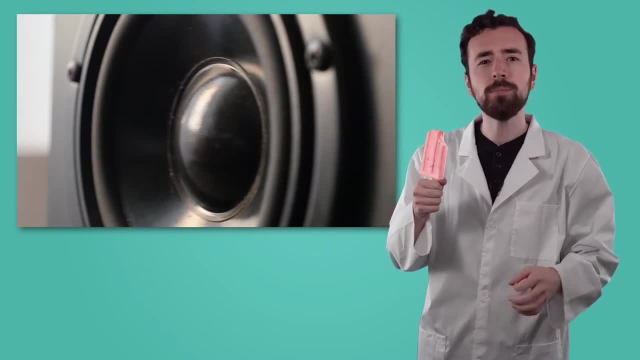 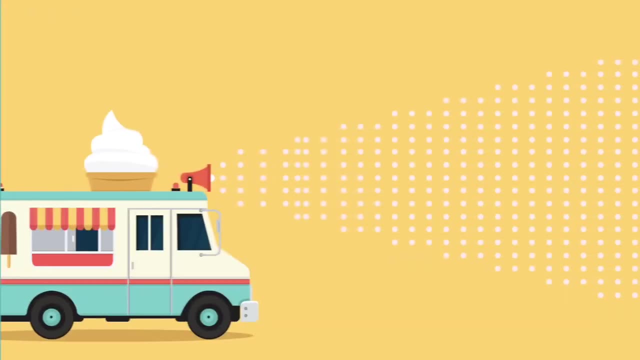 matter around the speakers to vibrate too. What matter is around those speakers, The air, As one particle of air vibrates, moving back and forth, it bumps into the next particle, causing that one to vibrate, knocking it into the next particle which causes it to vibrate, and on and on, like a 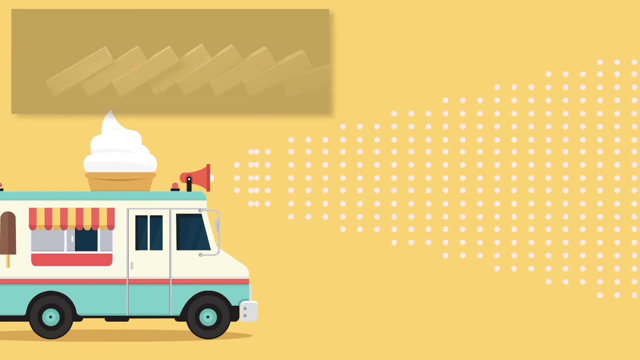 row of dominoes each knocking into the next. That chain reaction of air particles vibrating and bumping into the next particle which causes it to vibrate and on and on, like a row of dominoes, allows sound to travel great distances, including to my ears. 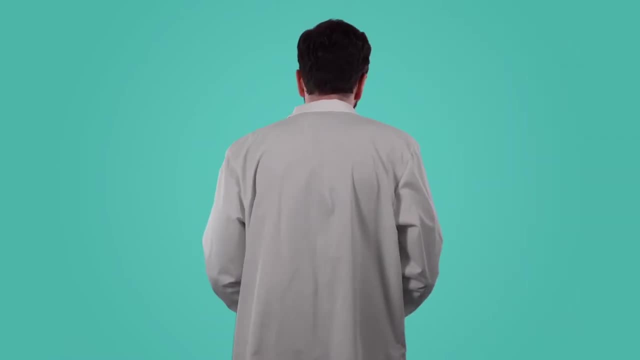 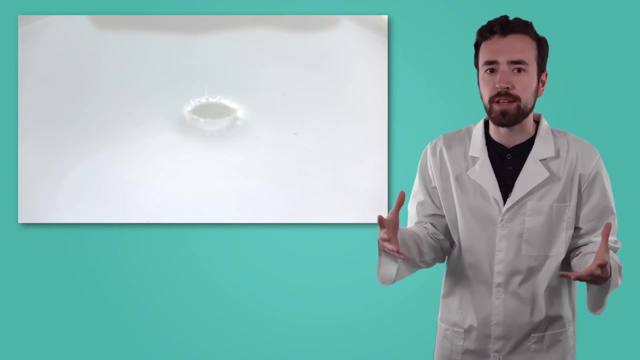 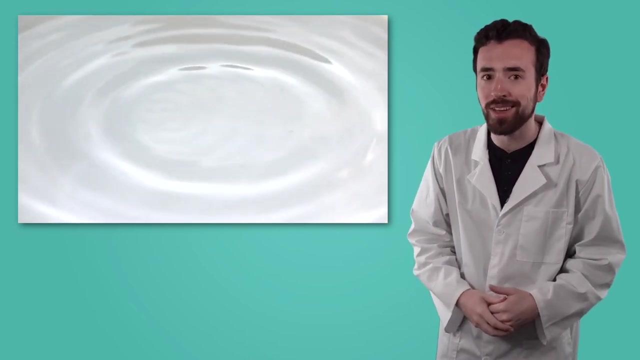 Sound doesn't just move in a straight line from the source to your ears, though. Oh oops. Sound vibrations move like ripples in a pond, expanding out in all directions from its source. That's why you can still hear someone talking, even if their back is to you. 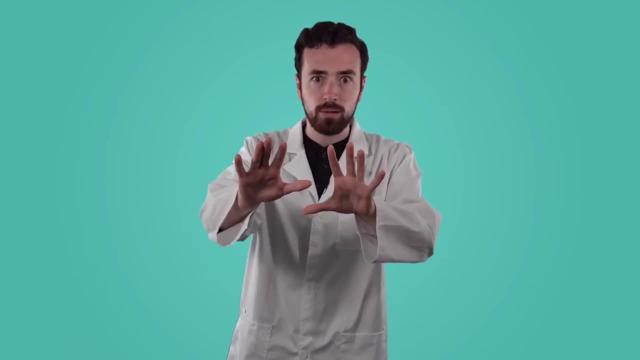 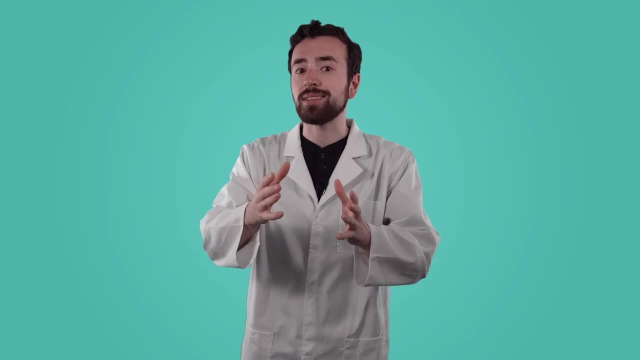 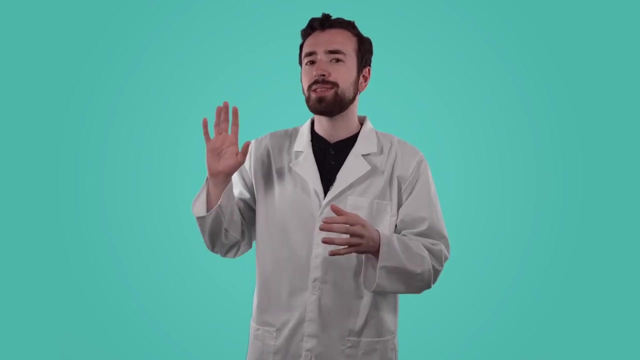 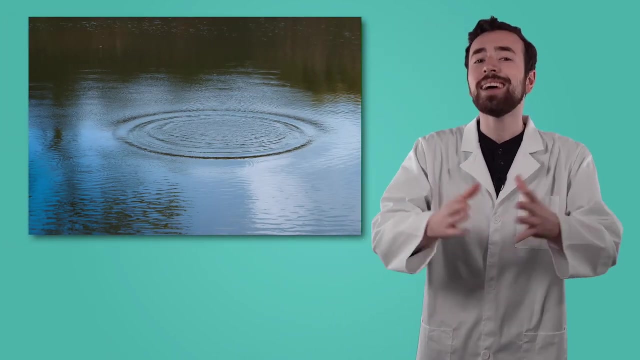 Wait, freeze. What sounds can you hear right now? You might notice that sounds with sources closer to you, like your device, sound nice and loud, But what do you notice about sounds that are coming from farther away, Also like ripples in a pond, as sound vibrations continue to move away from their source. 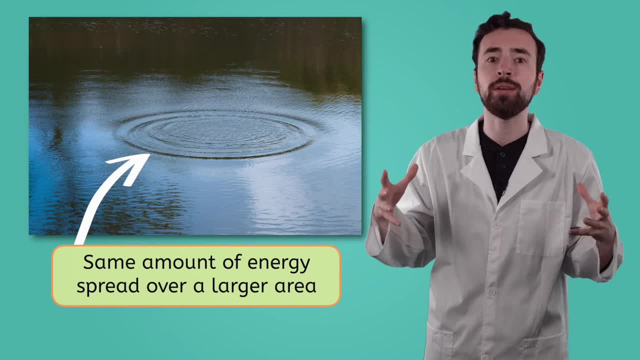 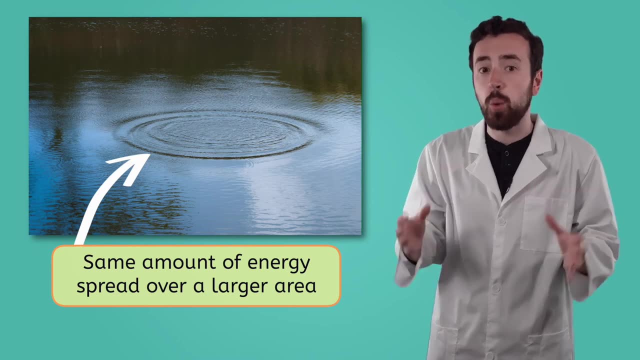 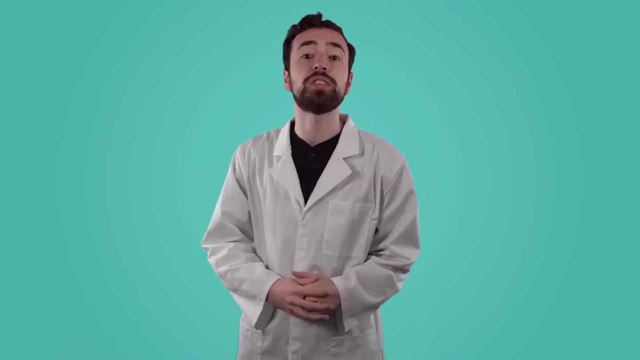 the same amount of energy is spread over a larger area. This means the sound is coming from farther away. The farther away from the source of the sound's vibrations you are, the fainter- or quieter- the sounds will seem. It's not only distance that affects how loud or quiet you perceive a sounds to be. 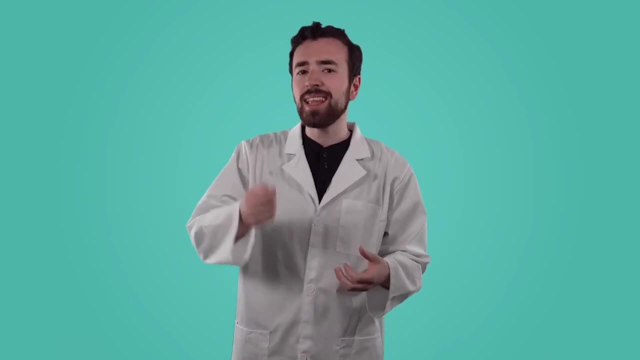 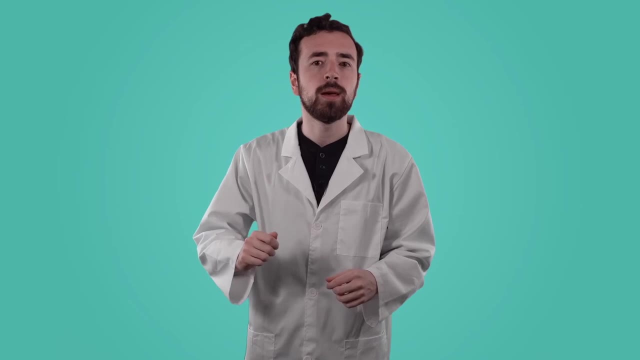 Try this out. Take a pencil and lightly tap it against your desk or a table. Listen to the sound it makes. Now, this may seem like a funny thing to ask of you, but try putting your ear on your desk, and when you crop it toward your side, it switches real quick. 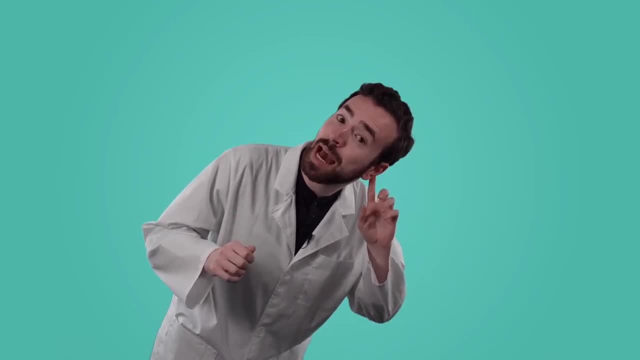 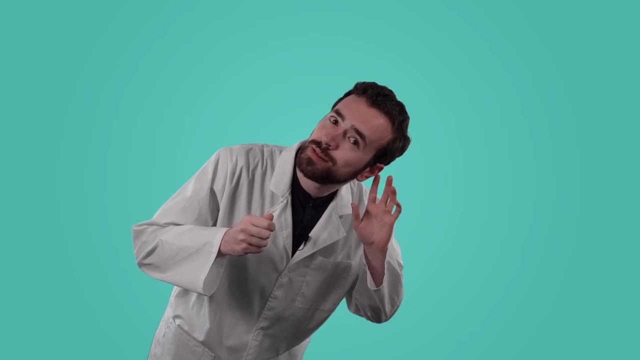 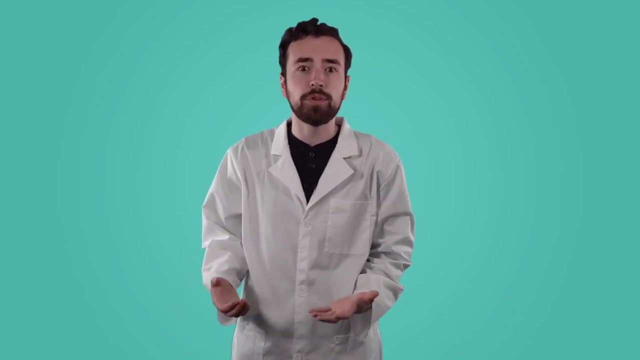 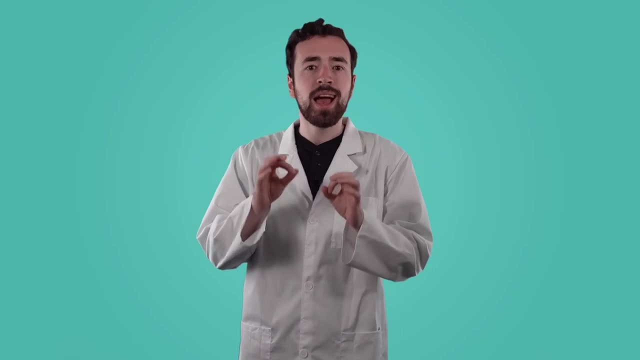 against the table's surface and then tapping the pencil again next to you. What difference do you notice? Uhhh, yeah, you gotta be careful with that one. You probably noticed that the sound of that tapping pencil got a lot louder, more like a hammer than a pencil. That's because sound actually travels. 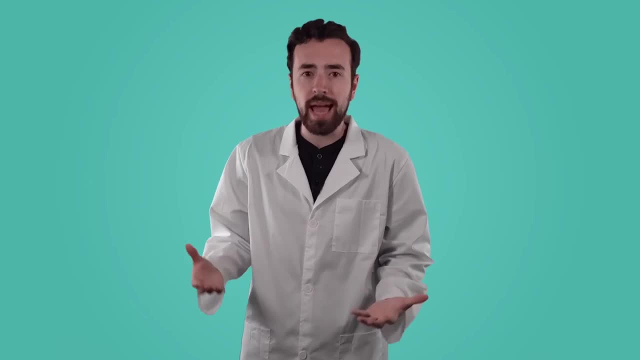 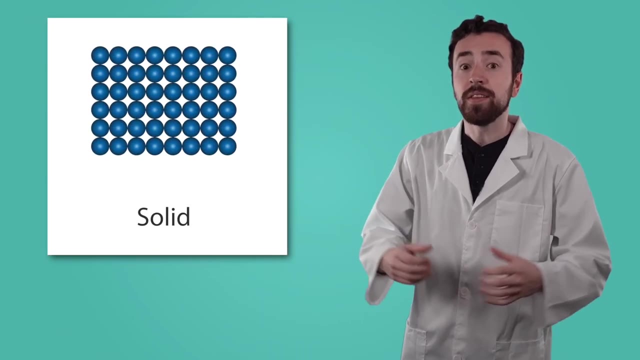 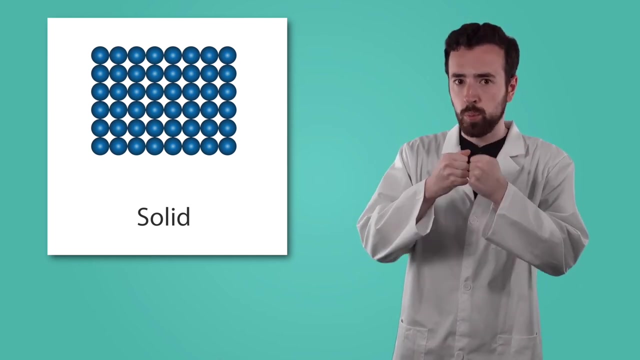 a lot faster through a solid than through a gas like the air. Do you remember the structure of a solid from our unit on matter? The atoms are packed tightly, super close together. Because they're so close together, when one atom vibrates it's able to knock into a lot of other atoms, super 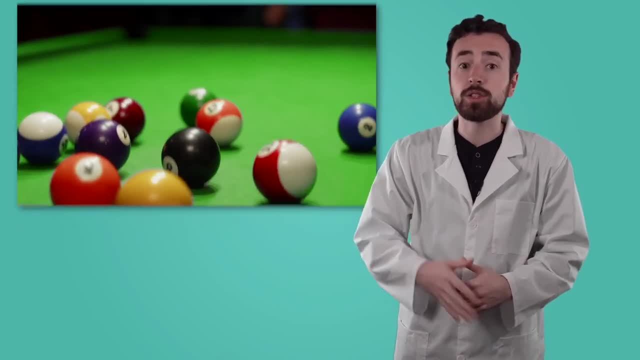 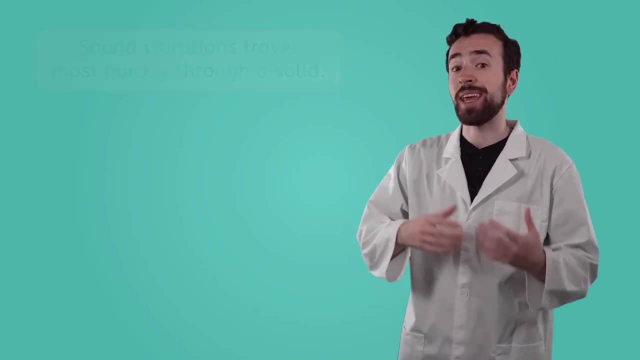 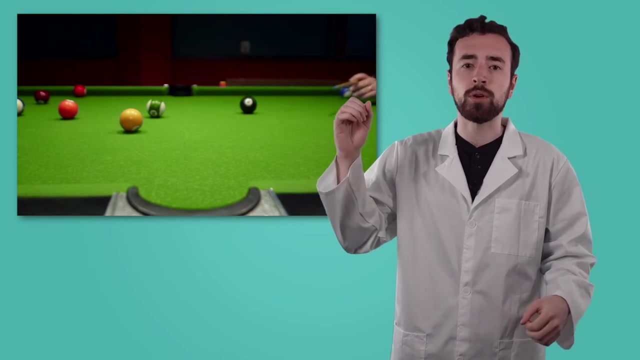 easily like billiard balls at the beginning of a game. So sound vibrations can travel very quickly through air. The atoms in a gas, on the other hand, are super spread apart, so it takes more time before sound vibrations cause one particle to bump into the next. Sound vibrations travel the most slowly.